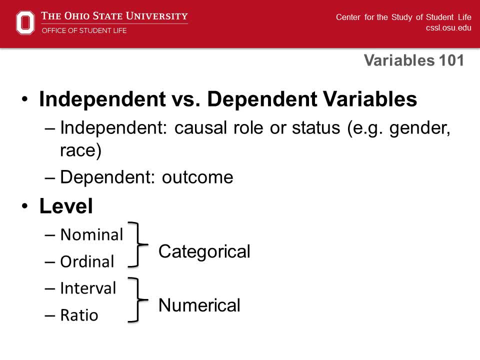 Variables are also characterized in terms of the levels of data they represent. Nominal variables consist of categories that cannot be ordered, such as gender or state of birth. Nominal variables are also mutually exclusive. This means that only one category can be true at a time. 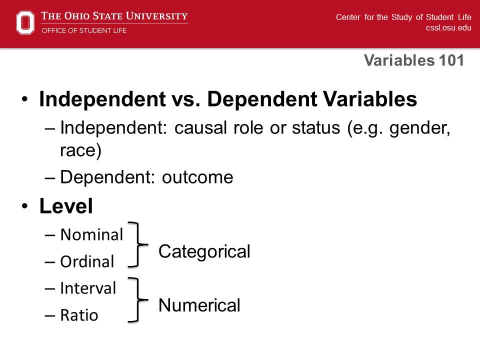 For example, a person cannot be both born in Ohio and Montana. Ordinal variables also consist of mutually exclusive categories, but there is a clear ordering of them. For example, if you ask someone to rate their health, and options include poor, fair, good and excellent. 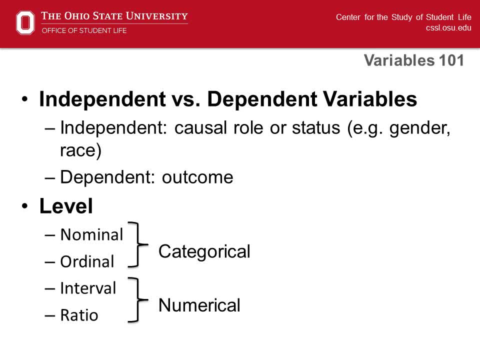 this is an ordinal variable. We can rank good health higher than fair health, but we cannot quantify the distance between those categories. Interval variables, on the other hand, have equal spacing between each value, such as with temperature. Ratio. variables are another type of interval variable, but they have a natural and meaningful zero point, such as weight or income. 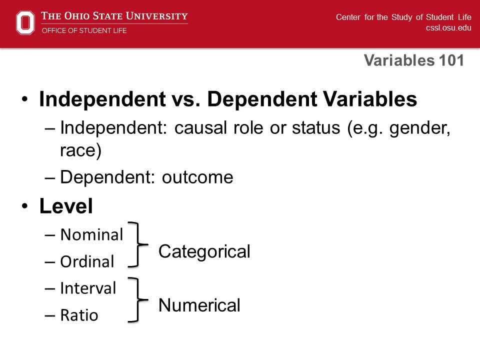 Nominal and ordinal variables are types of categorical variables, and interval ratio variables are numerical. In assessment work it is common to use Likert scales with ranges from strongly disagree to strongly disagree. Technically, a Likert scale is ordinal, but we often assign values from 1 to 5 to each answer option and treat data as an interval variable. 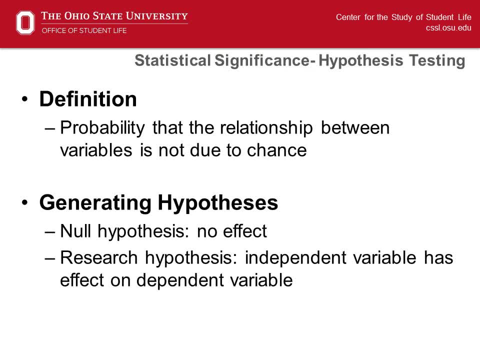 Before discussing which test you should run, we will explore the basics of statistical significance. Simply put, statistical significance is related to the probability that the relationship between your variables is not just due to chance. The first step in determining statistical significance is formulating your hypotheses about the effect your independent variable has on your dependent variable. 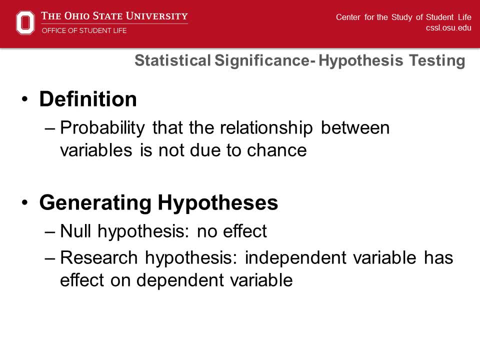 The null hypothesis suggests that your independent variable does not have an effect on your dependent variable, whereas your research hypothesis suggests that it does have an effect. An example of a null hypothesis would be students who participate in a student leadership program have the same graduation rates. 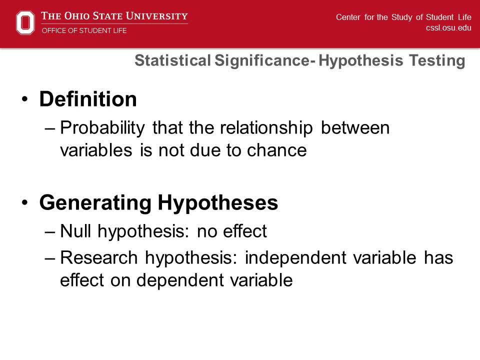 as students who don't participate in the leadership program. A research hypothesis for this example would be: participation in a student leadership program increases graduation rates. Please note that you can have one-way or two-way hypotheses. In a one-way hypothesis, you predict the direction of the relationship you are testing, as in the example previously mentioned. 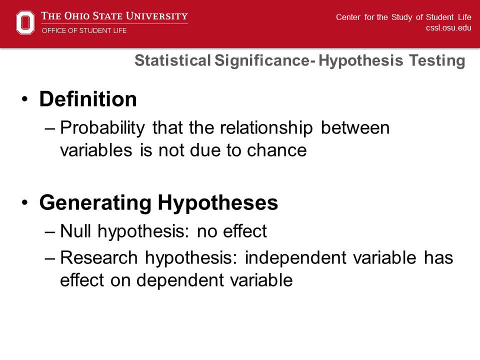 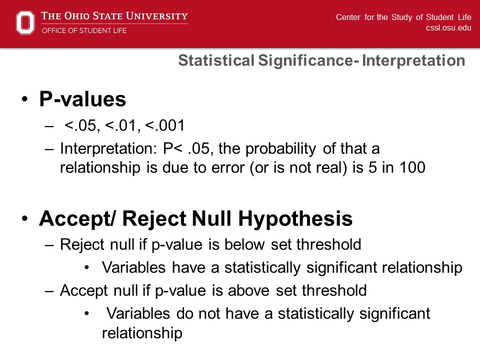 In a two-way hypothesis, you do not predict the direction of the relationship. In this webinar, we will refer only to two-way hypotheses, since we often cannot anticipate the direction of a relationship. Once you have your hypotheses, you can examine statistical significance using a p-value. 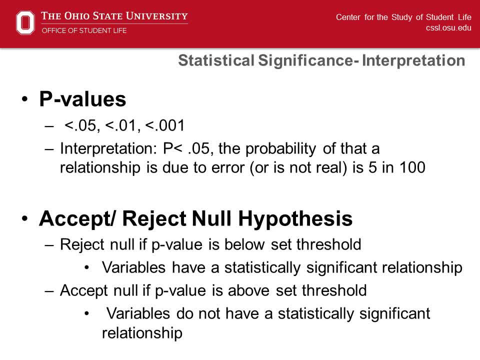 P-values refer to the probability that the relationship you find is real and not due to chance. Typically in student affairs, we consider tests with p-values less than 0.05 to be significant. A p of 0.05 means that a finding has a 5% chance of success. 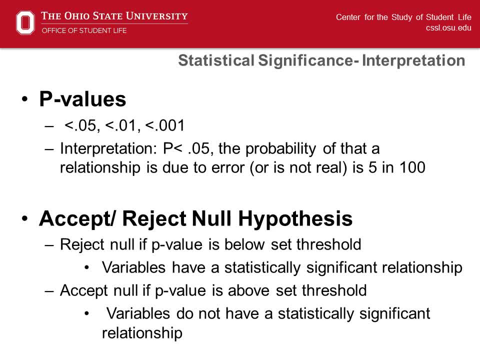 A finding has a 5% chance of not being true and a 95% chance of being true. For a p-value of 0.01,, this would be a 1% chance of not being true and a 99% chance of being true. 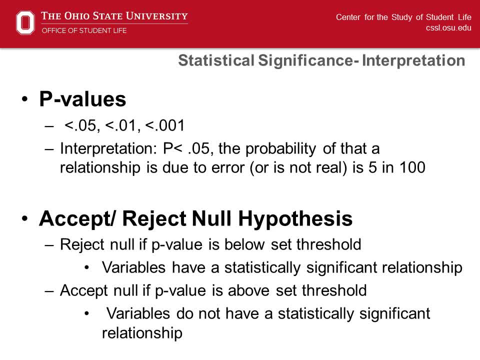 The smaller the p-value, the larger the significance, so the more confident you can be in your finding. If the p-value for your test is lower than 0.05 or your other predetermined value, you would reject the null hypothesis and accept the research hypothesis. 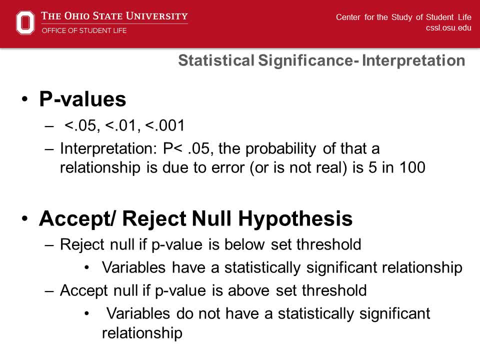 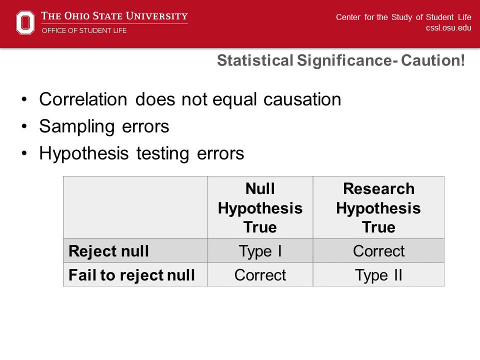 saying We have a statistically significant relationship. Let's say that we found a statistically significant effect on graduation rates for students who participate in a student leadership program. This means that the relationship of participation in the program to graduation rates is not just because of chance. 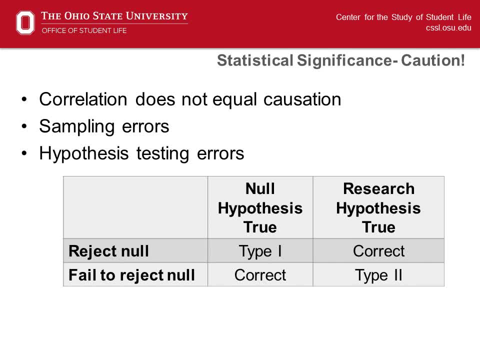 Although we can say the variables have a significant relationship, we cannot say that participation in the program caused the higher graduation rates. There could be other unobserved differences between participants and non-participants that influence their graduation rates. Determining causation is difficult. 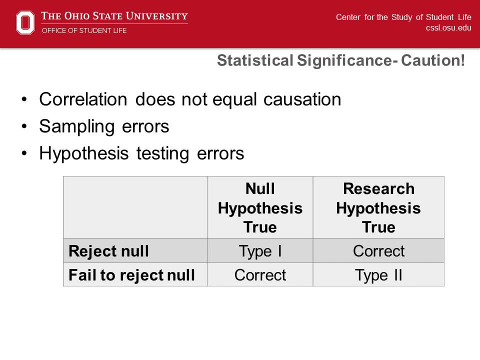 Typically you must be able to rule out other possible causes. The only way to truly rule out alternative causes is by setting up an experiment. When we do any sort of hypothesis testing we are assuming our sample is representative of the population. So in our example about the student leadership program, 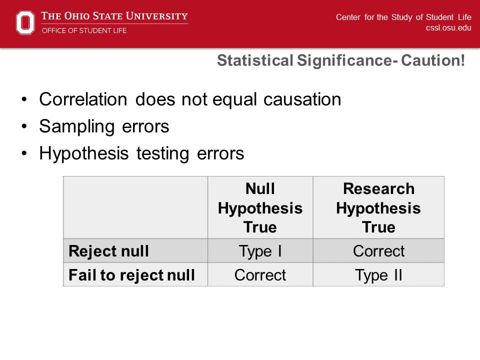 let's say we were only able to examine graduation rates for students who participated in a student leadership program led by one facilitator. If we looked at students who participated in the student leadership program led by all of the facilitators, it is possible that our results could be different. 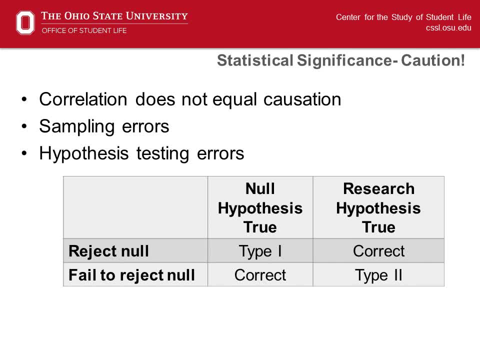 Much of the time, we weren't able to get data for the entire population we're interested in, So we have to accept that using a sample introduces error into our analyses. In addition, you should be aware of the two types of hypothesis testing errors. 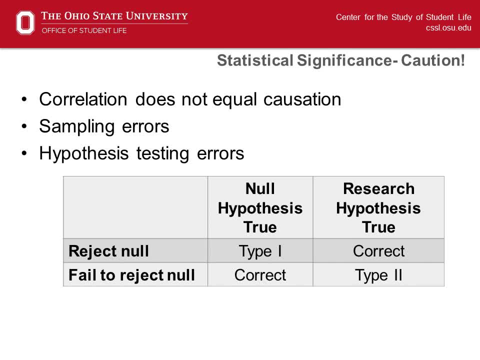 One type of error can occur when we decide to reject or accept the null hypothesis. Put simply, if you falsely reject the null hypothesis when it is actually true, you have a Type 1 error. If you fail to reject the null hypothesis when the research hypothesis is actually true, 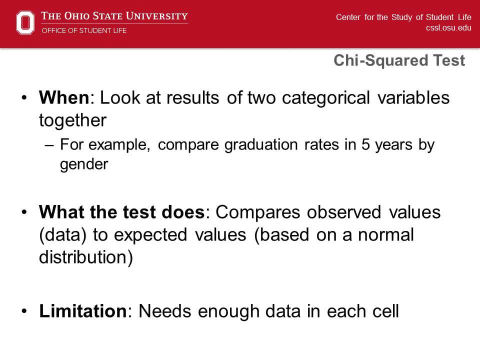 you have a Type 2 error. Now we are going to explore some commonly used types of statistical tests and explain when you would use each. The first test we are going to describe is the chi-squared test. We use this test when we want to look at the results of two categorical variables together. 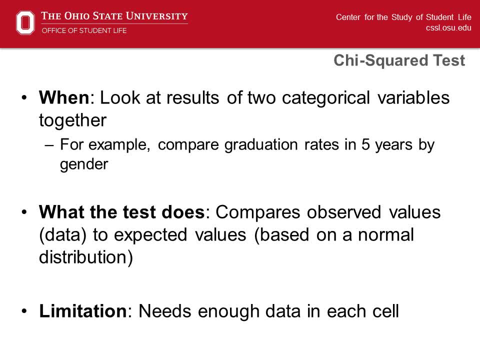 For example, we might want to examine satisfaction at an event by gender. Or, using our example of the leadership program, we might want to examine possible gender differences and graduation rates for students who participated in the program. The chi-squared test compares observed values for your data. 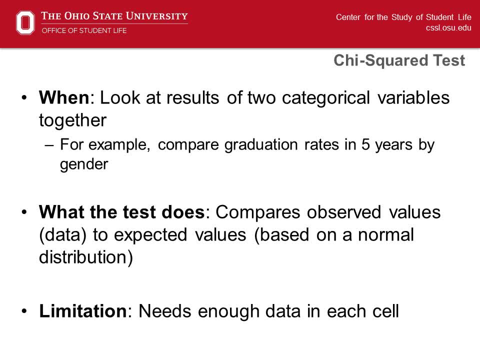 to expected values based on a normal distribution. Going back to our hypotheses, the null hypothesis would be that females and males who participated in the student leadership program would graduate at the same rate in five years. The research hypothesis would be that females and males in the program 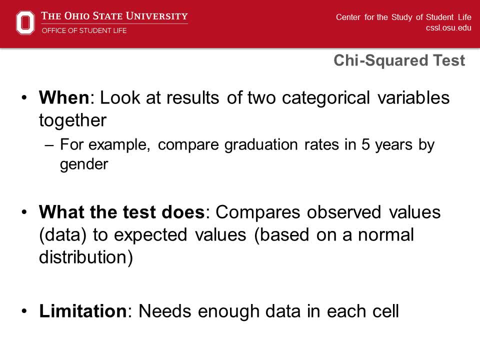 have different five-year graduation rates. Using the p-value from the test, you can determine if differences in the observed and expected proportions of males and females graduating are significant or due to chance. Chi-squared tests are a great tool for descriptive data. However, the test has some limitations. 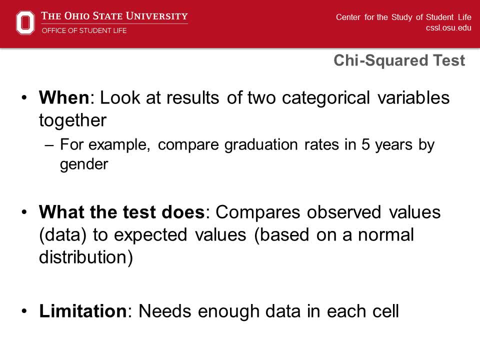 First, the chi-squared test is sensitive to sample size, meaning that large samples may be more likely to lead to Type 1 error. But if your sample or sub-sample you are examining is too small, you may not have enough data in each cell. 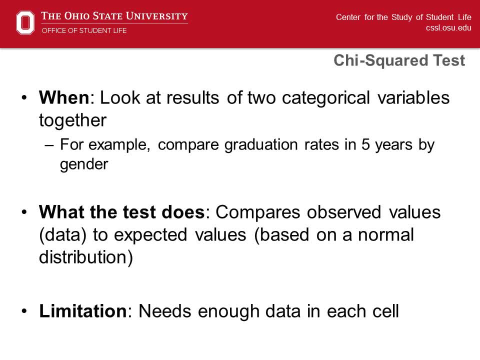 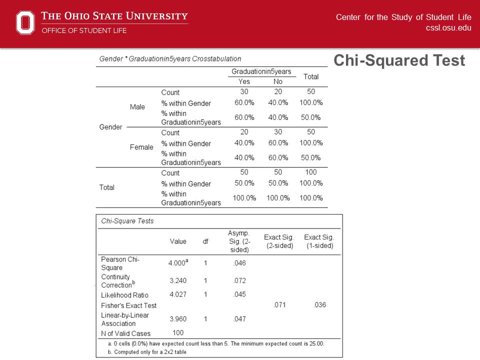 Also, the chi-squared test does not tell you the direction of the difference. It simply tells you that the values are different. This slide shows an output from SPSS for a chi-squared test. The first table: Graduation Rates by Gender- Cross-Tabulation. 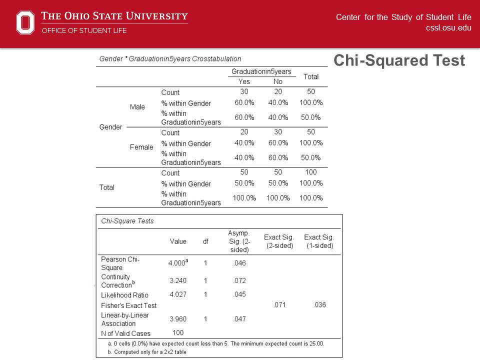 puts the percentages of graduation in five years In the table. you see 60% of males graduated in five years, compared with 40% of males who did not graduate in five years. In contrast, 40% of females graduated in five years. 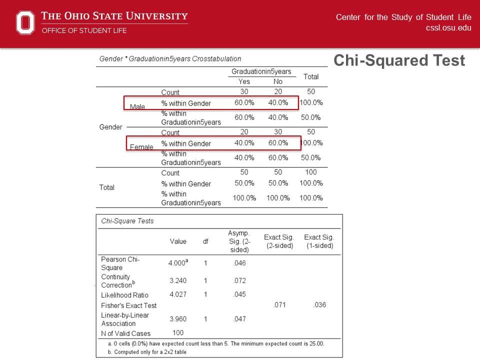 compared with 60% of females who did not graduate in five years. The second table shows the chi-squared tests and we will focus on the Pearson chi-squared rel. You want to look at the column labeled ASYMP SIG 2-sided. 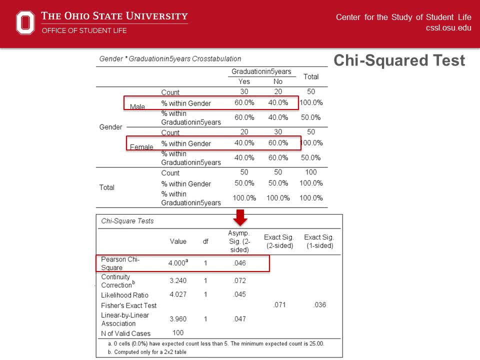 If this is less than .05,, then the chi-squared test is significant. For this example, it means that the proportions of females and males who participated in the Student Leadership Program and graduated in five years is not the same, and that this difference is likely not due to chance alone. 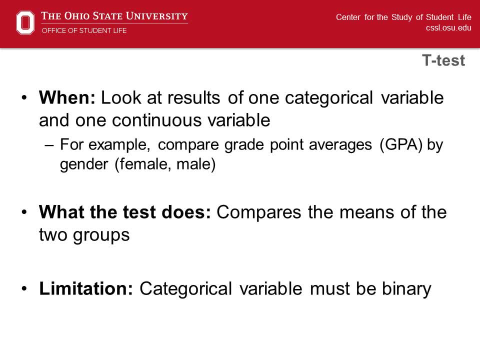 The next test we will cover is the t-test. You would use this test when you want to look at the results of one categorical variable and one continuous variable. The t-test compares the means of two groups, For example, if we wanted to examine if there was a gender difference in GPA. 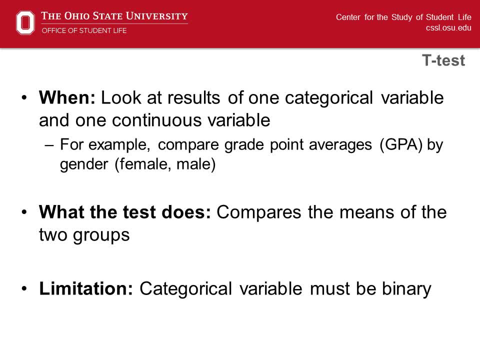 we would use the t-test. Going back to our hypotheses, the null hypothesis would be that there would be no difference in GPA between males and females. Our research hypothesis would be that GPAs differ by gender. Unlike the chi-squared test, the t-test tells you the strength and direction. 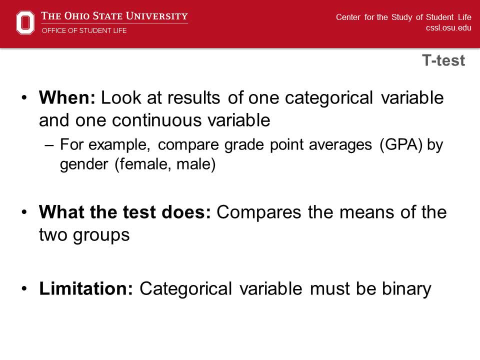 of possible differences in means. There are some limitations though. First, you can only compare two groups. Second, you can only examine the effects of one independent variable on one dependent variable. Another important point is that the best practice with this test is to have at least 30 participants in each group. 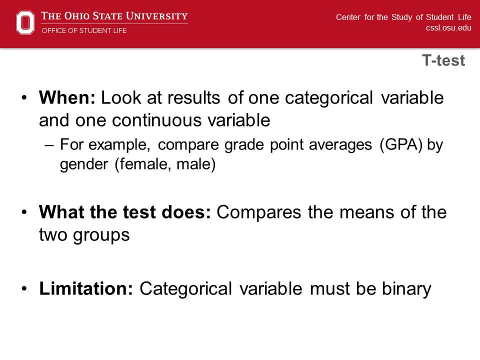 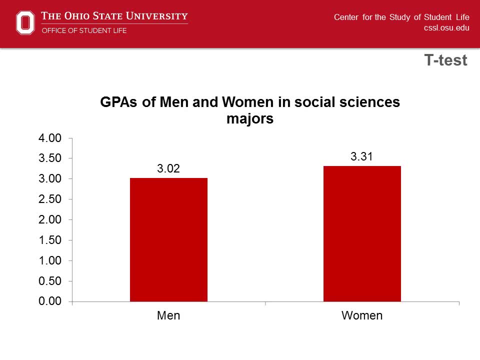 You can still do the t-test with fewer than 30 participants in each group, but you would be less certain of the results. This slide shows the two means without any indication of significance. Based on this graph, it appears that women have higher GPAs compared to men. 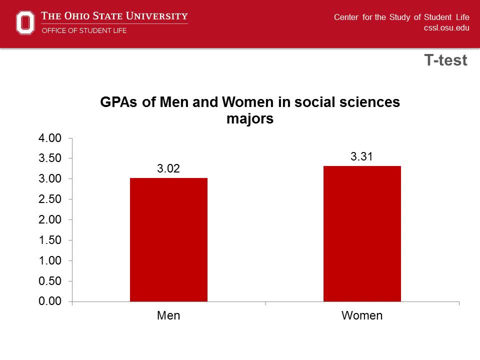 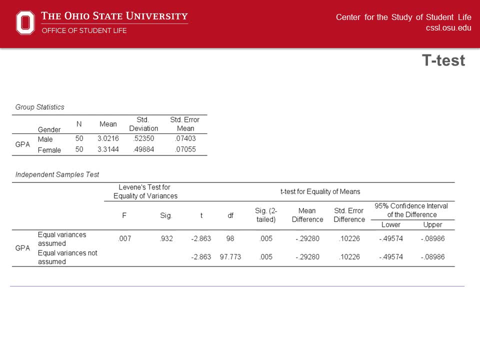 but we should also look at the t-test results to determine if this difference is statistically significant or due to chance. Here is a sample output for the t-test. First we examine Levine's test for equality of variances. It tells us which row of the sig. two-tailed column to look at. 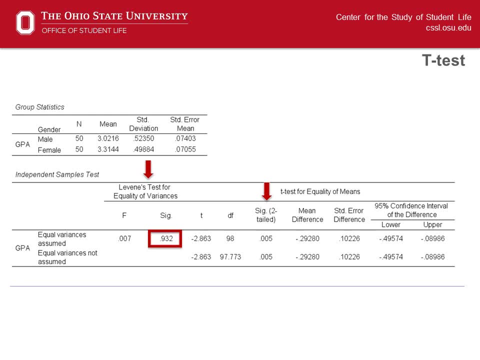 If the p-value for Levine's is above 0.05,, then we read from the first row. If it is below 0.05, then we read from the second row. Now, looking at the top row of the sig two-tailed column: 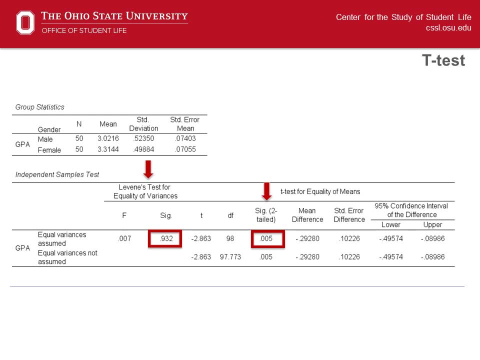 we can determine statistical significance, It is 0.005, so we should reject the null hypothesis because 0.005 is less than 0.05.. This implies that there is a statistically significant difference in GPA between men and women. We could also examine GPA differences for a variety of demographic variables. 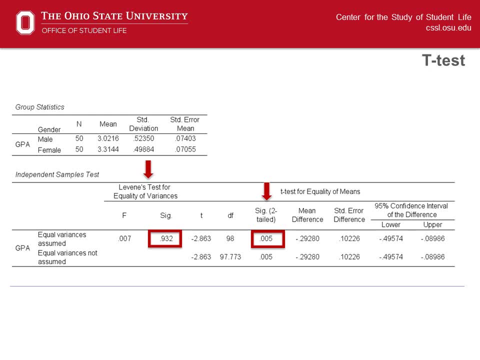 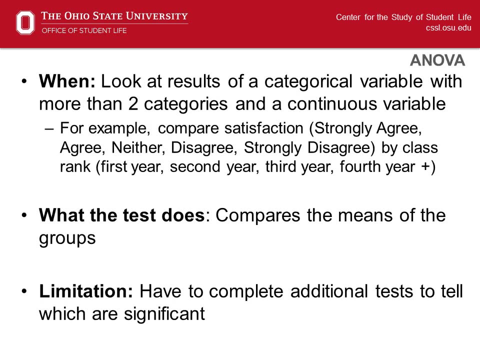 but for a t-test. they have to be grouped into two categories, such as white and non-white students or first-year and non-first-year students. The final test we will discuss is the ANOVA. We use this test when we want to look at the results. 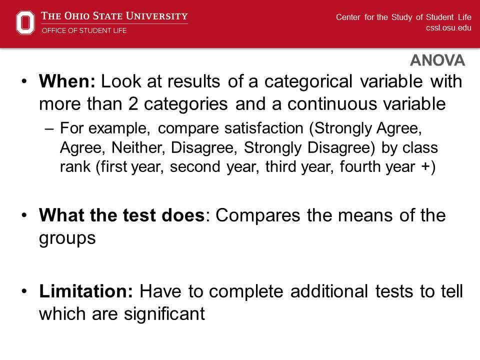 of a categorical variable with more than two categories and a continuous variable. The ANOVA test compares means of multiple groups. For example, let's say we want to compare GPA by class rank. Our research hypothesis would be that GPA differs by class rank. 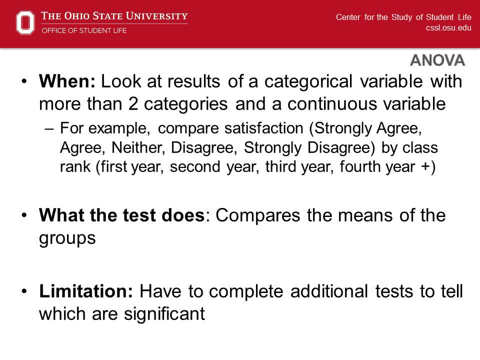 and the null hypothesis would be that there is no difference in GPA by class rank. There are some limitations to the ANOVA test. The test only tells you if the means of your groups are significantly different from each other In order to find out which means score is significantly higher or lower. 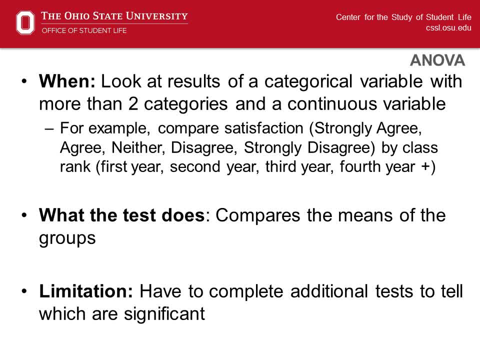 you need to perform additional post hoc tests. These can be selected when you run the analysis in the statistical software program and are discussed in more detail in the resources provided at the end of the webinar. This slide shows the average GPA for each of the class ranks.